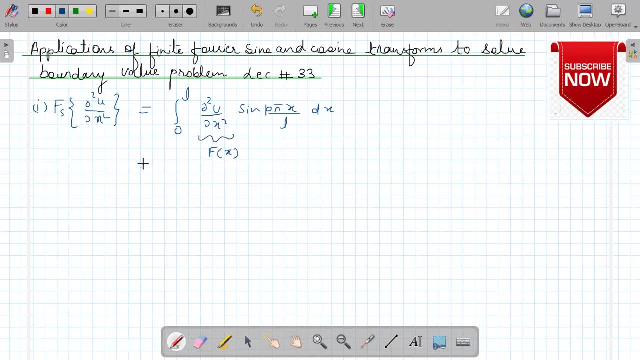 the function f x. Okay, So we integrate this by parts. First function: This is our first function And this is taken as second function. So first function into integration of second function. So we write first of all del U by del x, and then we write sine p, pi, x over L, Then we apply a limit in this part Minus. 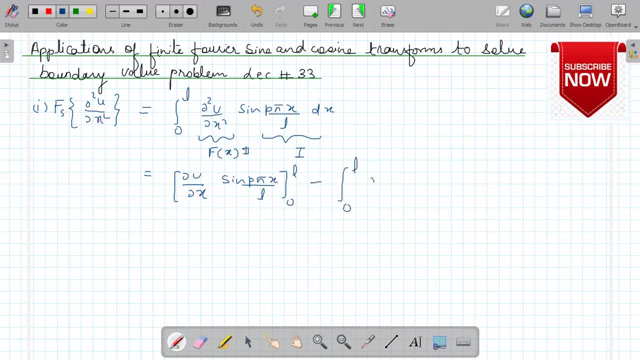 integration zero to L del U by del x, cos, p, pi, x over L, dx. Okay, So this is finite. Fourier sine of x over L, differentiation of this And the extra part which is in denominator, which is p, pi upon L. it will become sorry in, not in the denominator, it will in the 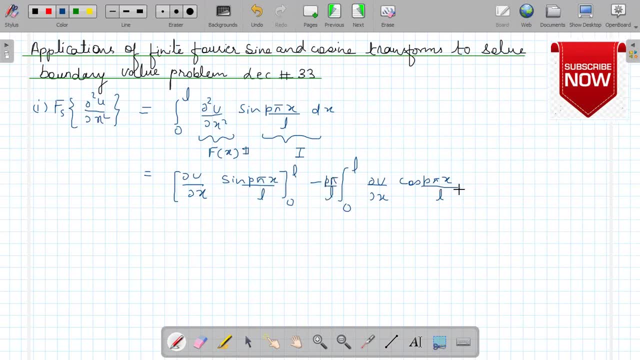 multiplication. So we have p? pi over L, because we are differentiating this function. So we have f over L, We are differentiating the potentials. then we have p? pi by L, So we have x over L. So we have a time pinch which is one exponential and we are differentiating. 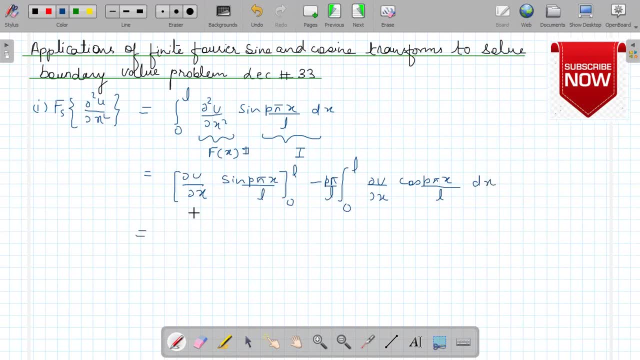 So we assume that del u by del x. we don't know the value of del u by del x at the upper limit, So we write this as it is. But when you substitute l here you will get sin p, pi, which is 0, and at lower limit this is automatically 0. So this whole term vanish, Yeh pura term. 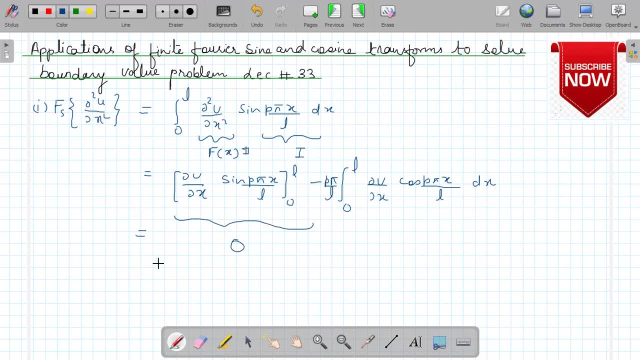 zero ho jayega. What is left is this: So we have minus p pi over l u x comma t cos p pi x over l 0 to l minus integration of u x comma t cos p pi x over l u x comma t cos p pi x over l 0 to l minus integration. 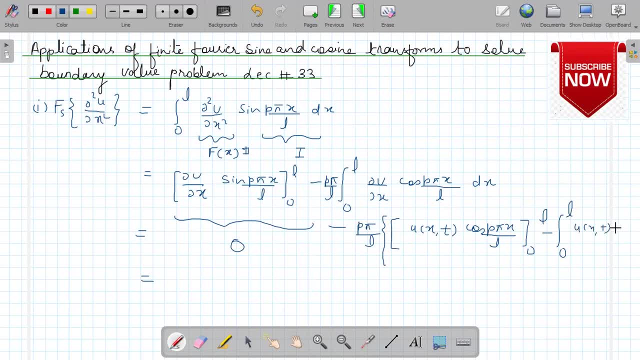 of u x comma, t cos p, pi x over l u x p, because the derivative of course is negative, So we have positive sign here: sin p pi. Let me write this expression in the next line, because in the next line, because it is not coming in this line, So let me write it again. 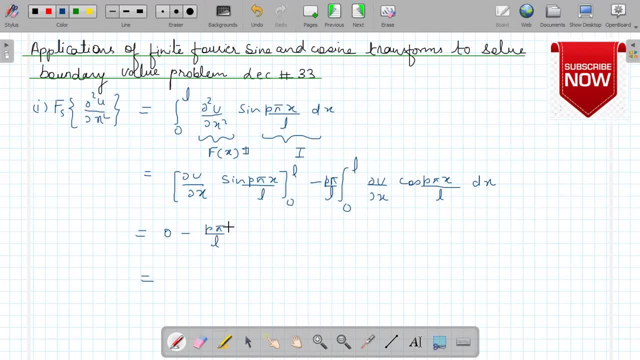 p pi over l? u x comma. u x comma t? u over l? u x comma t. cos p pi x over L, minus 0 to L? u x comma t, sine p pi x over L into p pi over L. so we have minus p pi over L. 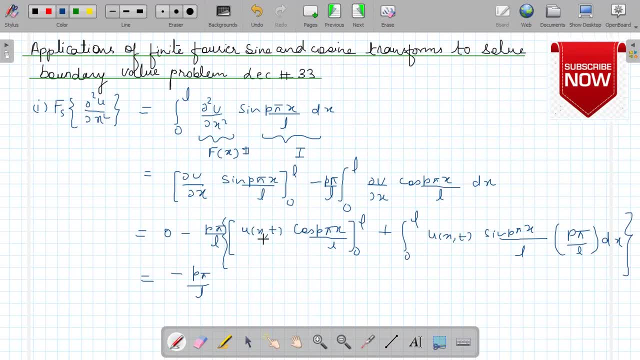 u L comma t and cos p pi is minus 1. raised to the power p? u L comma t and at lower limit, this will be 1 and we are left with u 0 comma t. okay, and here we have p minus this, p pi over L. 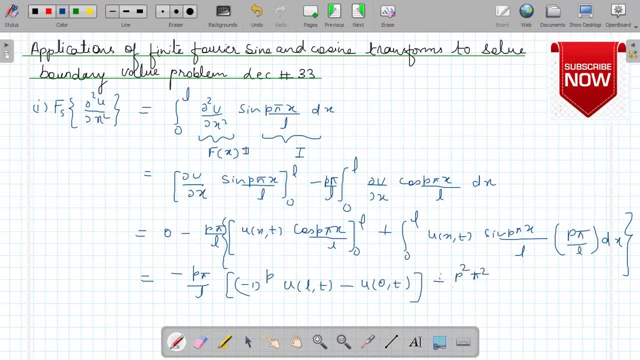 will get multiplied with this p square, pi square over L square and this integral. if you see it carefully, this is Fourier sine finite, Fourier sine transform of the function u, which can be denoted as u s bar. okay, so you see here that we need the value of u. 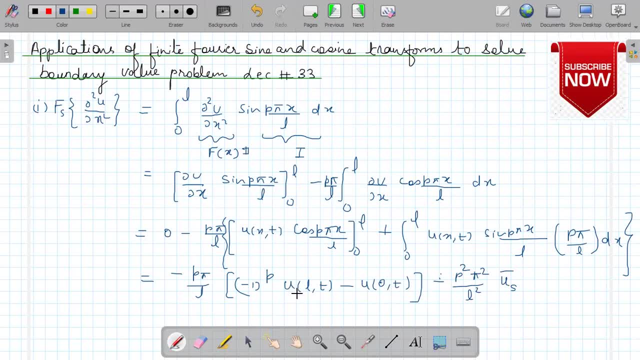 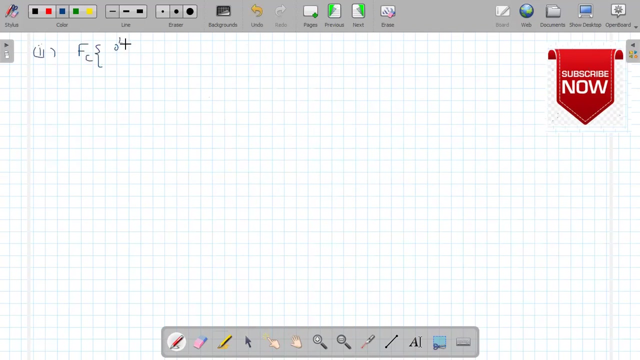 at 0 comma t and L comma t. these two are needed to solve this. okay, so this is the what happened when we apply Fourier sine transform to the second derivative equation. let's see what happened when we apply Fourier cosine transform in the same differential equation. this is 0 to L. 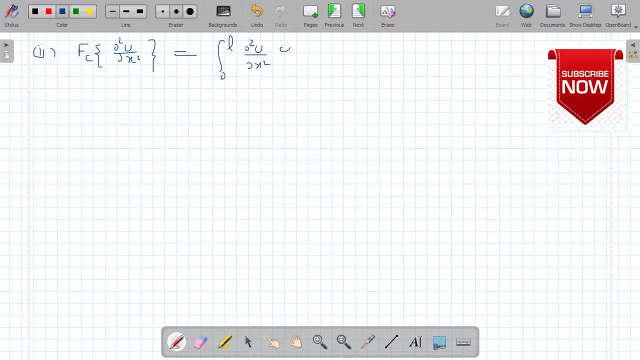 del 2? u over del x square cos p pi x over L minus 0 to L del 2? u over del x square cos p pi x over L px. again we use chain. sorry, integration by parts del by del x cos p pi x over L. 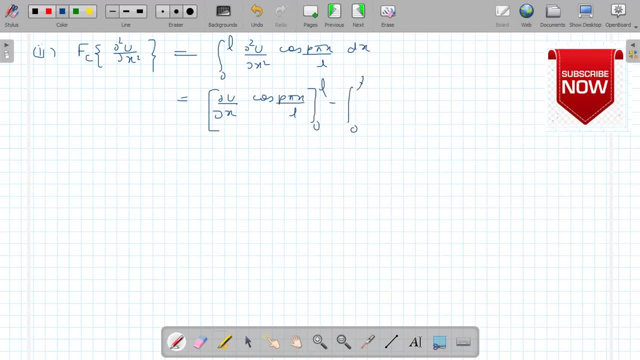 0, 2 L minus del u by del x sine p, pi x over L into p, pi over L over L px. this is- you can denote this by ux, L, comma t at, when we substitute L at the place of x and cos of p, pi is minus 1 raised to the power p at lower limit. 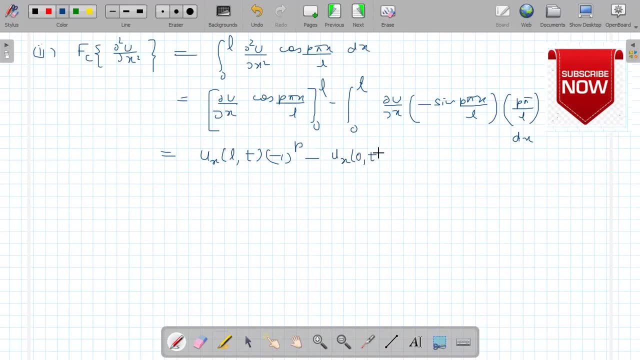 this will be ux at 0 comma t and this is minus minus plus p pi over L, integral 0 to L del u by del x sine p pi x over L gx ux L comma t. this means del u by del x value at L comma t. okay, this is not mu, this is u. 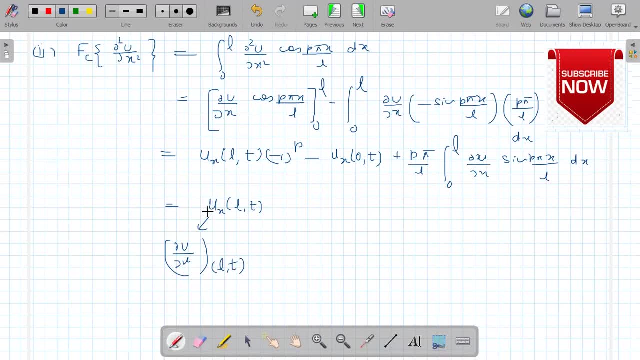 this is u minus 1 raised to the power: p minus ux 0 comma t plus c pi over L ux comma t differentiation. sorry, integration of this and this function as it is 0 to L minus integral ux comma t. differentiation of sine p pi x is cos p pi x over L into p pi over L dx. 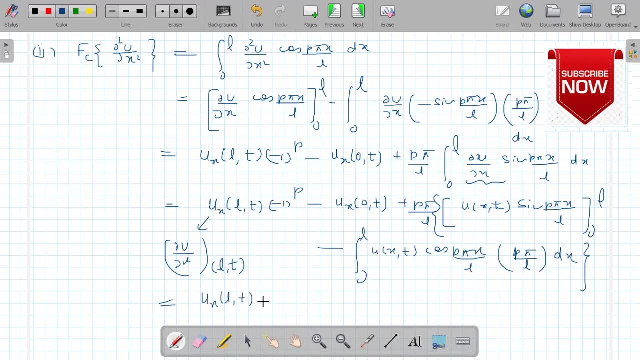 you x L comma t minus 1, raised to the power p minus ux, 0 comma t. certeza 5 0 0 0, 1 0, 1 0, 1 0 0 0 that we have P square, pi square over L square, and this integration is nothing but Fourier. 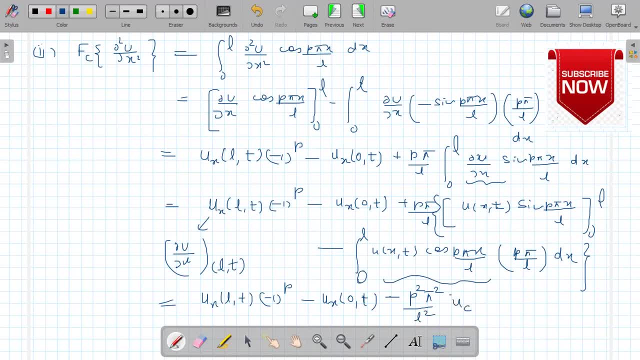 finite Fourier, cosine transform, the function U that is denoted by UC bar. So you see that we need the derivative value at 0 comma T and L comma T. So this is the hint that you have to apply, whether sine transform or cosine transform, If you are given the derivative. 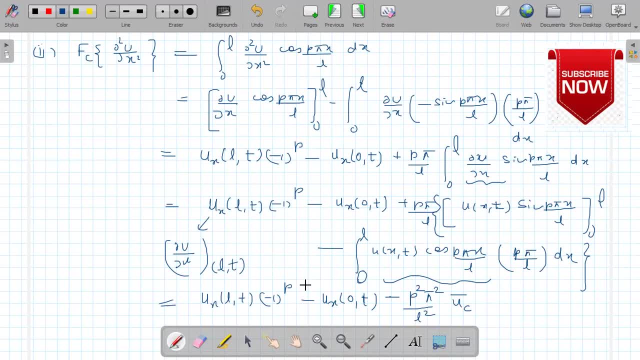 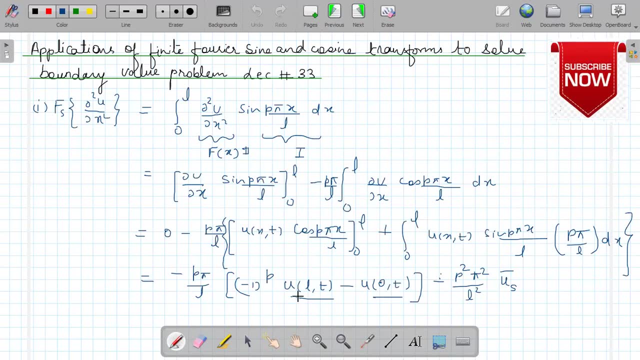 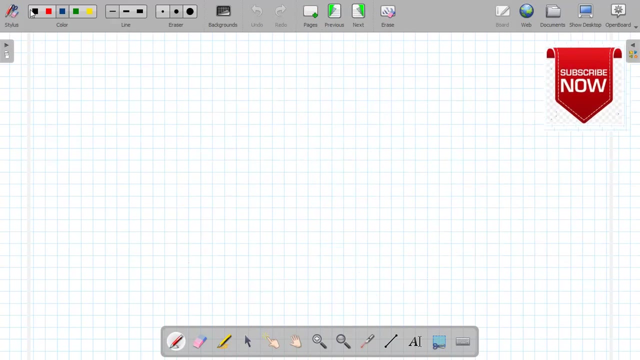 value at 0 and L, you apply Fourier cosine transform. If you are given the value of U at 0 and L, you will apply Fourier sine transform. So let's see one example: Solve del u by del t is equal to del 2 u over del x square, where x lies between 0 and 4. 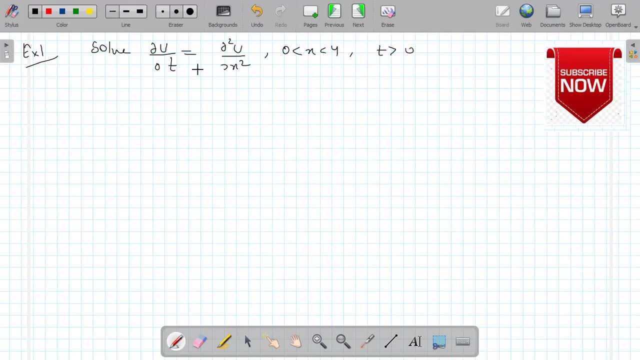 t is greater than 0, such that u 0 comma t is 0 and u 4 comma t is 0 and u x comma 0 is 2x. so as you can see, the here that limit of the variable is from 0 to 4. 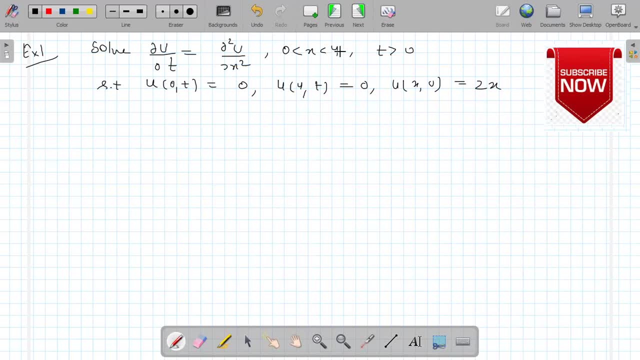 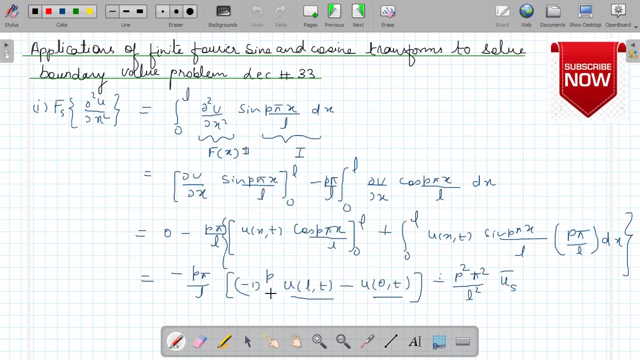 which is finite. so we will apply here finite Fourier sine or cosine transform. now, since the value of u is given at 0 and 4, which is required, as you can see here, 0 value of u at 0 and L, which is required when we apply Fourier sine, 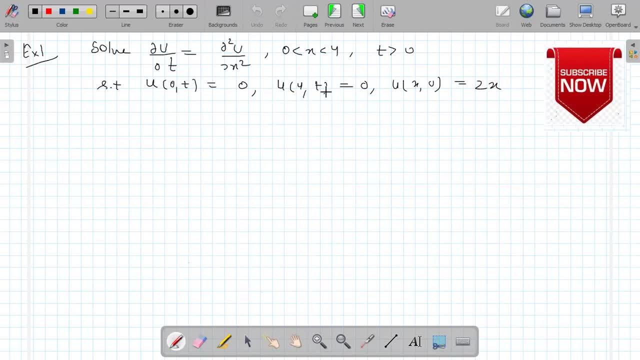 transform. so these two values are given to us. that means we will apply here Fourier finite Fourier sine transform. okay, so let we are given this equation: del u by del t is equal to del 2 u over del x square. so we apply here finite Fourier sine transform. 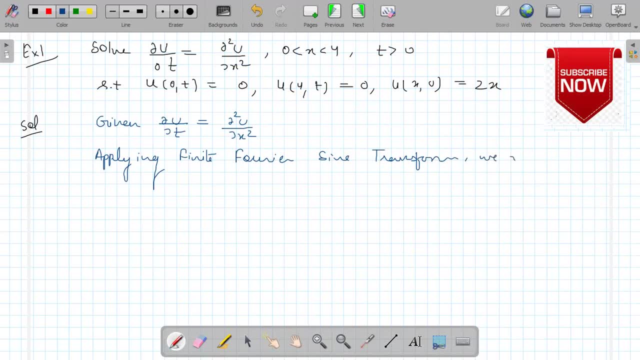 we get 0 to 4 del u by del t sine p pi x over 4. 0 to 4 del 2 u over del x square sine p pi x over 4 DX. now, since this derivative integration is with respect to X and this derivative is: 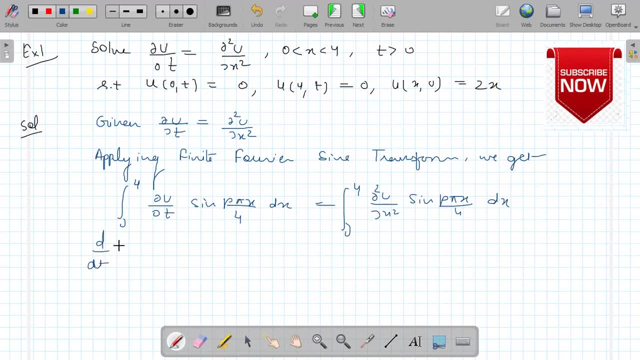 with respect to T. so this can be written as T over DT of 0 to 4, u, x, comma, T sine p, pi, x over 4 DX. and here we apply integration by parts rule del u by del x. we take this as first function and this as second function, first function into integration of second. 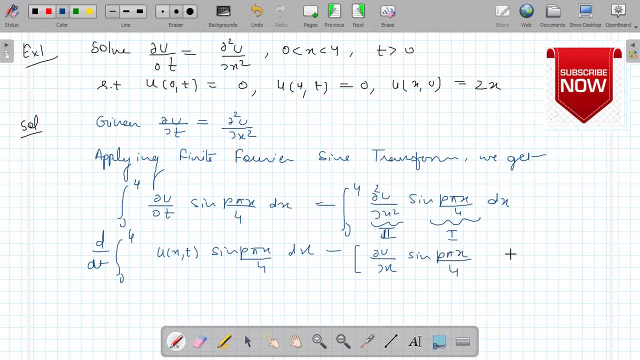 function integral del u by del x, cos phi upon x P Pi over 4 will come outside vx 0 to 4. so and here we apply integration by parts rule del u by del x over 4, we take this as first integral del u by del x and this as first function into integration of second Mo. 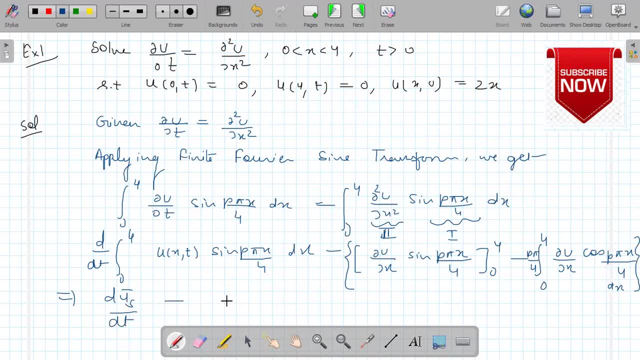 Copilot, also neighborhood, so this can be written as P. pi over 1 minus 1 sole integral del u by del X c exp I have a source for x is equal to total integral del u minus. this. will be 0 at both limits and this will be. 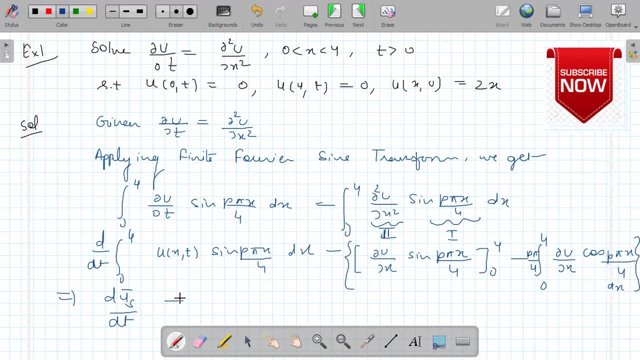 plus E pi over 4, ux for Marty or E pi X, X over 4 and limit 0 to 4 minus these P pi over 4. integral 0 to 4 for ux for Marty. sign P pi X over 4 because the derivative of course is: 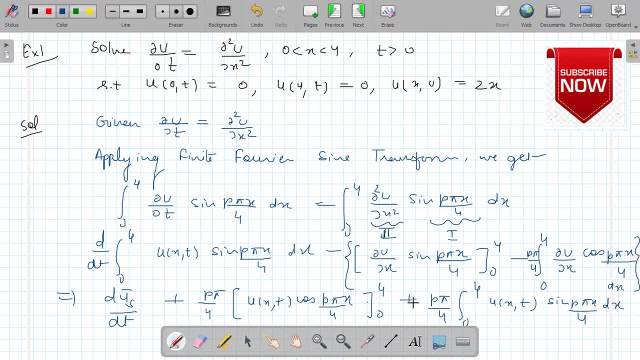 negative, so we have positive sign here. this is equal to sign. I'm sorry, so that' and this is like this. okay. so we need the B radian. this is like okay. we need the value of B radian group of P费, P b and. 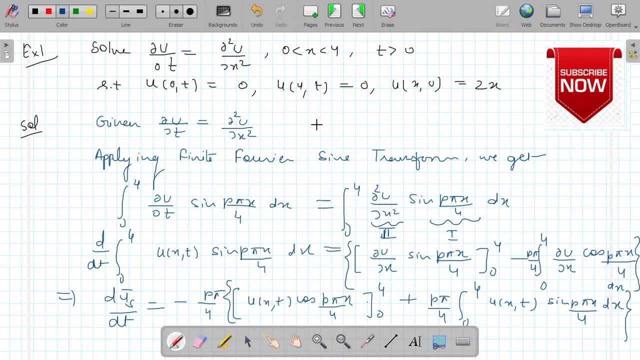 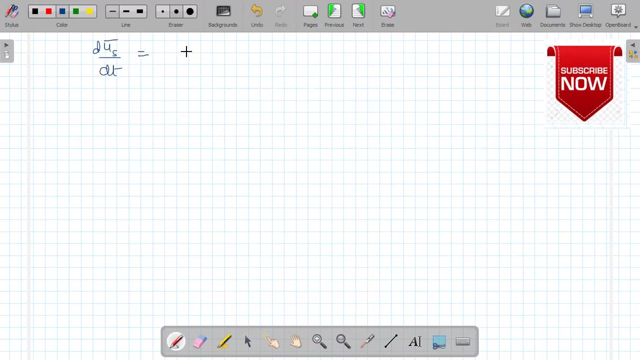 yes, so M value of U 4 comma T, which is 0, and at lower limit this will be U 0 comma T, which is also 0, so this whole term vanish and we are left with D? U S bar over D T is equal to minus. 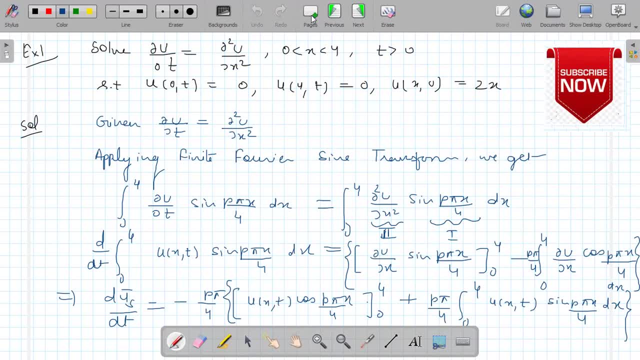 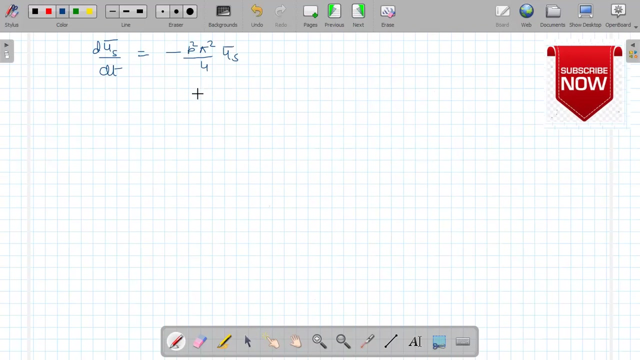 P square, pi square over 4, and this expression is nothing but U S bar. okay, so, so this is also four square. now we are given we can separate the variables. P? U S bar over U S bar is equal to minus. P square, pi square over 16 D T, so that we 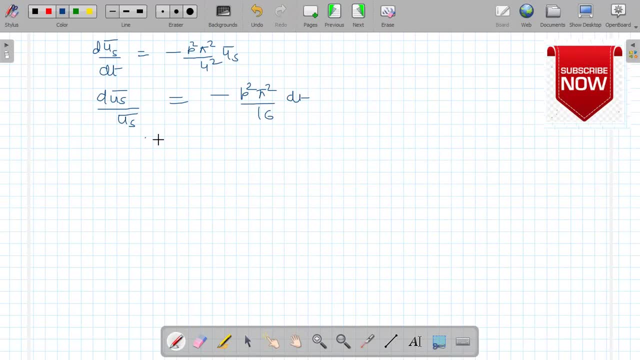 have log of U S bar is equal to minus P square pi square over 16. P plus log of C. this implies U S bar is equal to C, e to the power minus P square pi square square over 16 into T. okay, where C is constant. so this is nothing but U S at P. 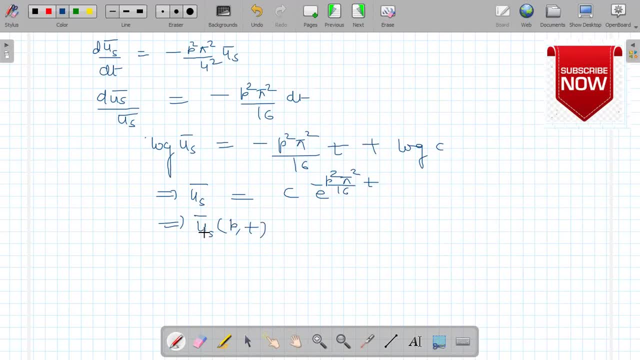 comma T. this is C e minus P square pi square over 16. when we put T is equal to zero, we have U as bar, P comma 0 because we have T here, so we can put T is equal to 0, we cannot. put P is equal to 0, we cannot. 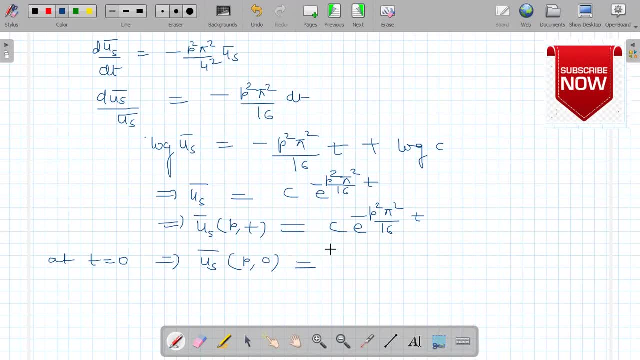 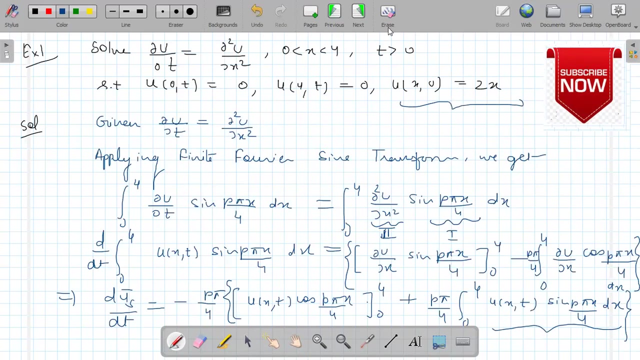 put T is equal to 0, we cannot put P is equal to 0, we cannot put T is equal to 0, be 0, because we have two variables here, x and t. so we can put t is equal to 0 so that we have c. so we need the value of this. so for this you are given in this condition, u. 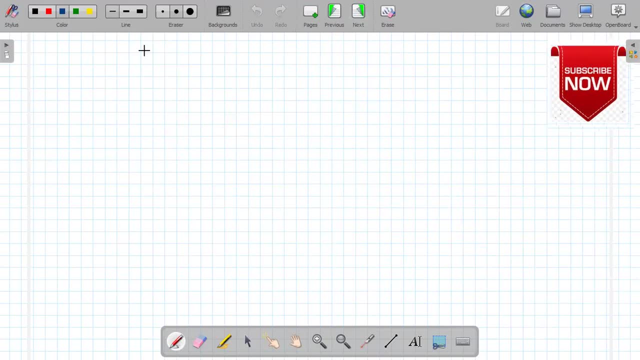 x comma 0 is equal to 2x. so u x comma 0 is equal to 2x. so that we take the finite Fourier sine transform of this and we have 0 to 4, 2 x sine t x comma. u x comma 0 is equal to 2 x, and we have c of f and u x comma 2x and all of these. 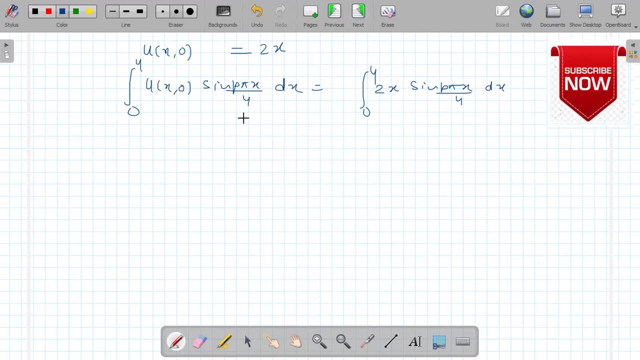 pi x over 4 b x. this is denoted by u s bar x, p comma 0, because after solving it you will get the function of p. so we will replace x by p and it is equal to we solve this first function. integration of second function, minus derivative into integration again. 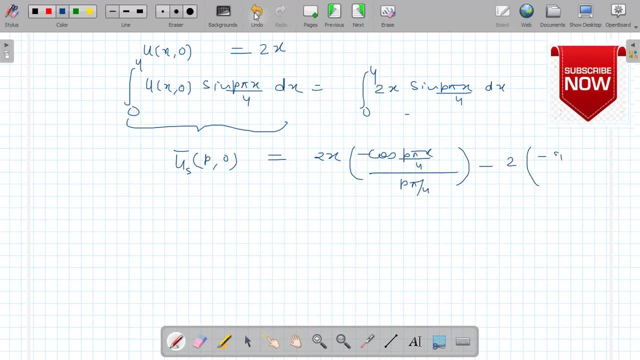 sine and we will get the function of p. so we will replace x by p and it is equal to. we solve this first function integration. again, sine p, pi x over 4 over p square, pi square over 60 supply the limit. so we have 8 x over p pi cos, p pi x over 4 plus 32 over p square. 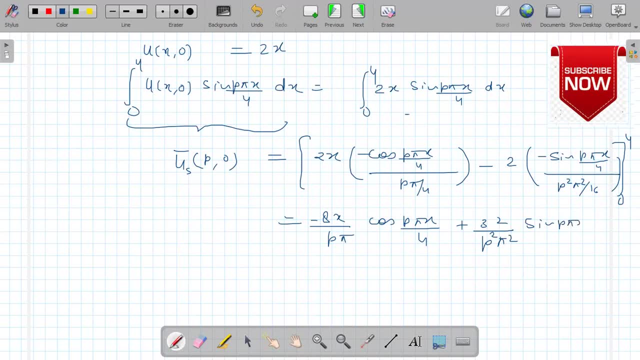 pi square sine P PI X over 4. now we apply the limits so we have minus 32 over P PI into minus 1 raised to the power P. and because force of P PI is minus 1 raised to the power P, the sine P PI is 0 and up at lower limit both will be 0. so we have this 32. 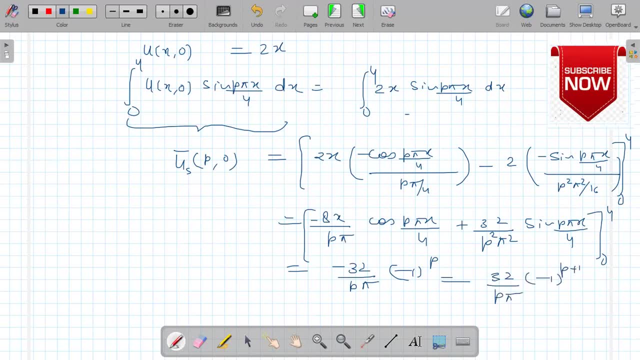 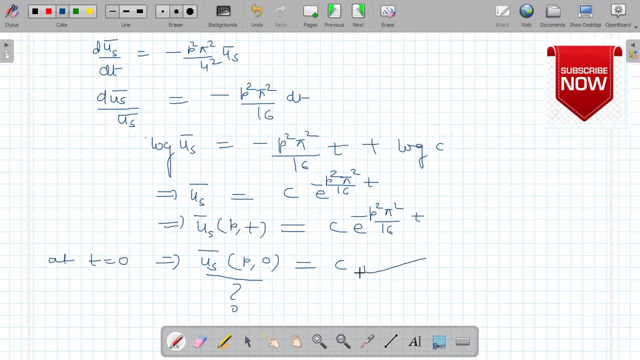 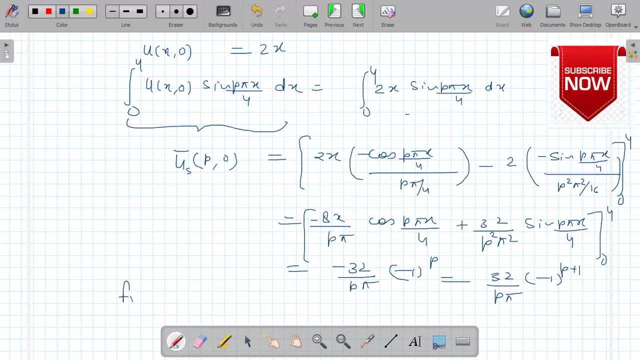 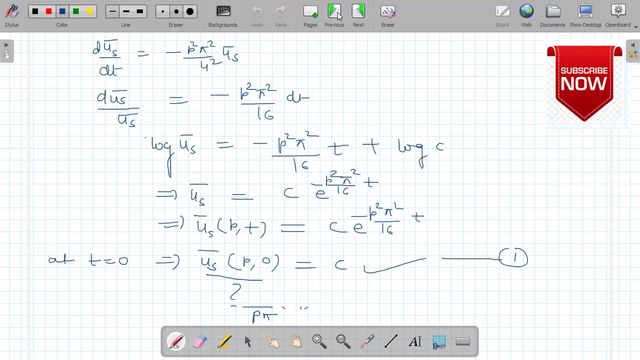 over P PI into minus 1 raised to the power P plus 1. so we substitute this value in this equation. so from 1, C will be 32 over P PI minus 1 raised to the power P plus 1. this is the value of C. now we will substitute the value of C. 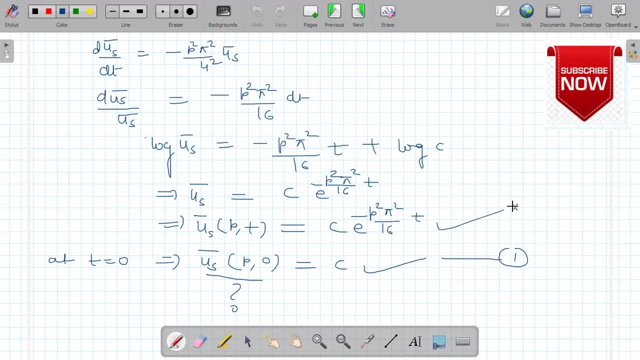 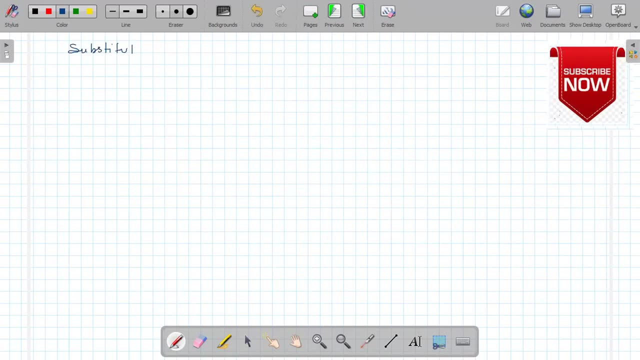 here in a star, substituting the value of C in a star, we get US P comma T 32 upon P. PI minus 1 raised to the power P plus 1. E raised to the power minus P. square PI square over 16. this is F as of U X comma T. okay, so next step is to take inverse finite Fourier sine. 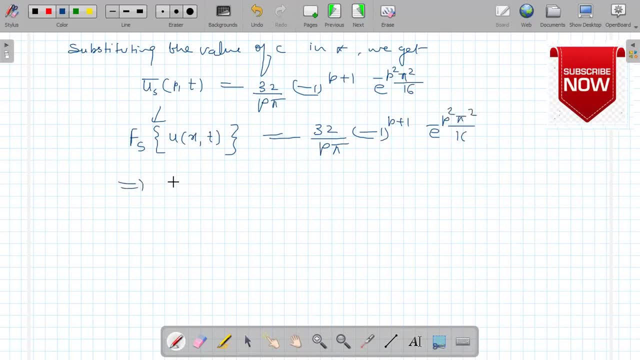 transform of this expression U, X comma. T is F as inverse of this whole. okay, you, so UX committee is, by definition, it is 2 upon L, which is for summation. U S, p, the point E sine P, PI, X over 4, we have 1 upon 2 of 32 upon p pi, so we can take 32 upon pi outside, so that we have 16 upon pi. 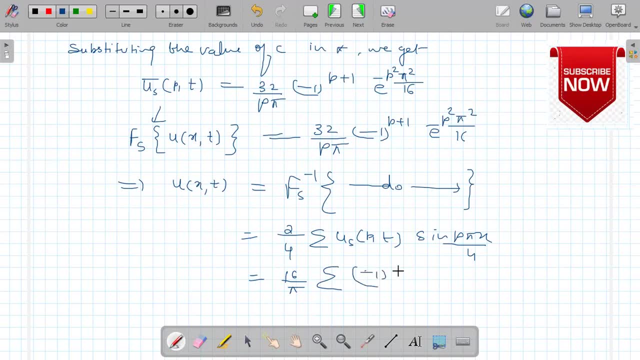 summation: minus 1 raised to the power p, plus 1 over p. e raised to the power minus p. square, pi square. this is t also. I have skipped this. yes, we have t here also, t over 16 into sine p, pi x over 4. 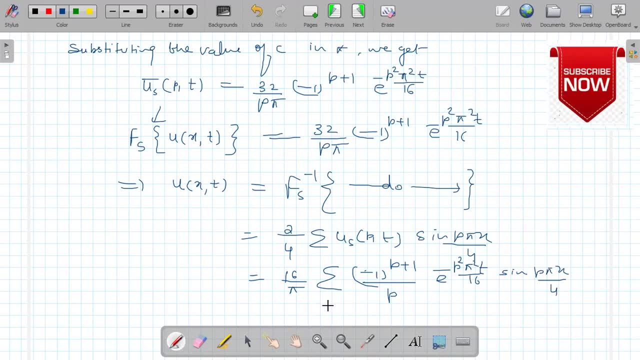 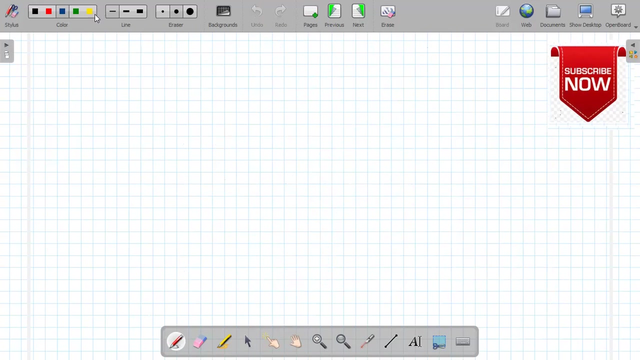 this is the answer where summation is over p and the summation varies from, I think, 1 to infinity. okay, so we leave it here. this is the answer. next move on the second example. second example is one ici. so second example is to solve del u by del t k, del 2 u over del x square, such that del u by del x is 0 when. 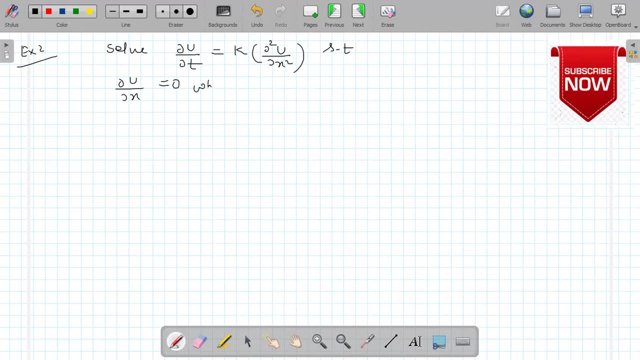 x is equal to 0 and x is equal to 5. both are equal to 0. t is greater than zero in both cases and u is not zero. c is 0 is a function of X at t is equal to 0. this is initial condition. X varies from: 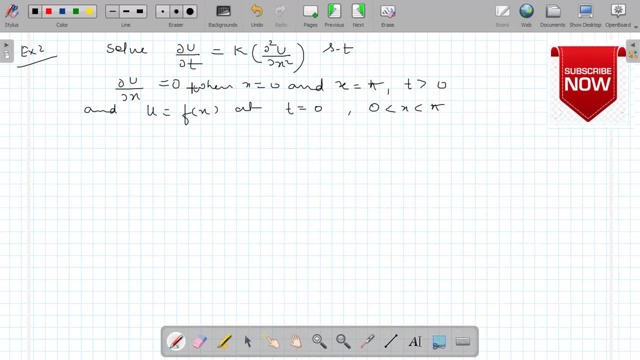 0 to 5. these are the boundary conditions. this is the boundary condition and this is the initial condition. initial condition will be a time t is equal to 0, per, given out here a boundary condition. the boundaries for X- you know boundaries and per function key value. care for your value, given out here that. 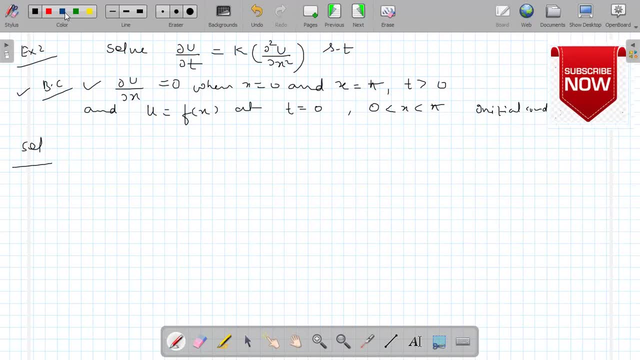 is boundary condition. so you key. obviously you are given the derivative value at the boundaries. so we apply Fourier cosine transforms, Fourier finite, Fourier cosine transforms on the given equation. so limit is from 0 to pi del u by del t cos px, because L is pi dx. 0 to pi K del 2 u over del x squared cos px dx. 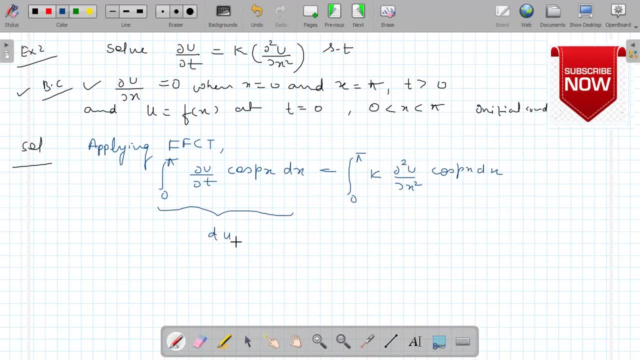 so we write this as du C bar over DT, and here we apply integration by parts rule. we always take this as first function and this as second function. we have here P, and because the derivative of cos is negative, so we have positive sign here. sine P, X, P x, the derivative value at pi is 0 and at at X is equal to 0. this is again zero. so the full term is zero. so that whole, so this whole term is: 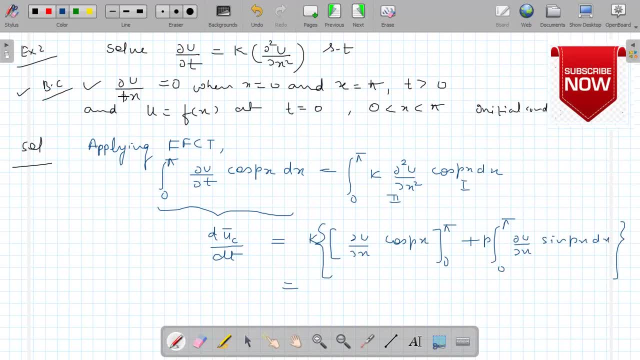 zero, 0.. So we are left with k into p. We will give the reason here why this term is 0.. Okay, I am not mentioning here kp again. we integrate this by parts: ux, comma, t, sine of px 0 comma. 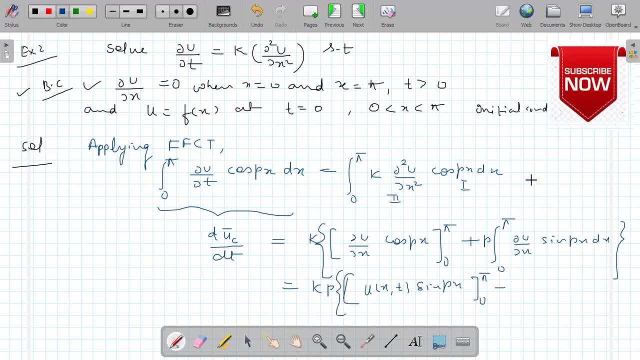 pi minus integral ux, comma t, cos, px, tx. Okay, So we again this whole will be 0 at upper limit as well as at lower limit, because sine p, pi is 0 as well as sine 0 is 0.. So this: 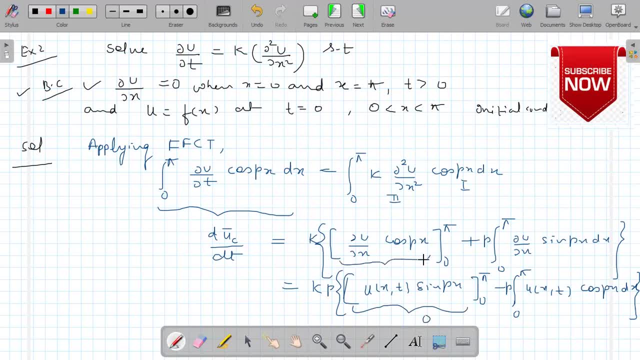 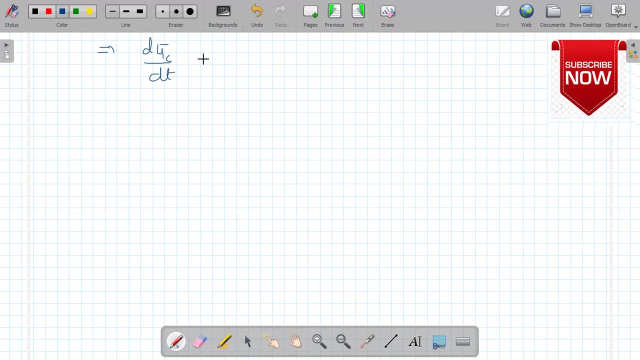 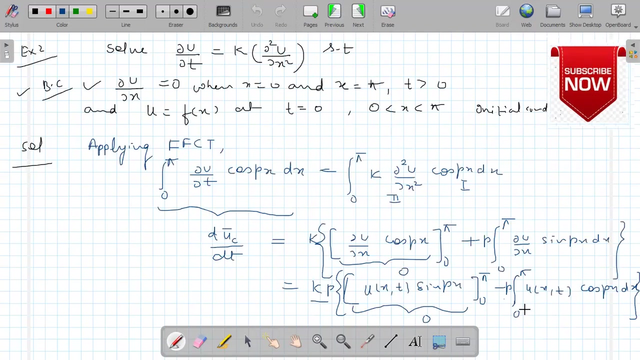 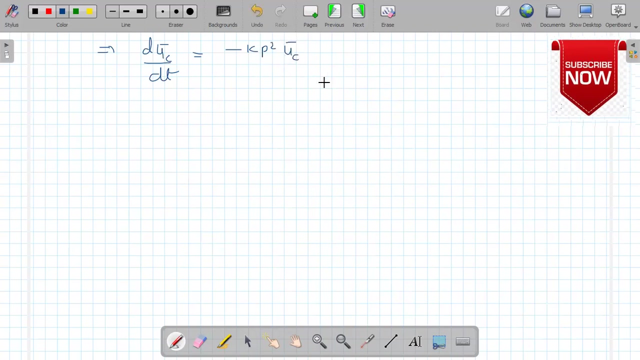 will be 0.. You should write the reason why they are 0.. Okay, So we multiply this kp with this p so that we have duc bar over dt is equal to minus kp square, and this is nothing but for finite Fourier cosine transform of the function u, which is denoted by uc bar. 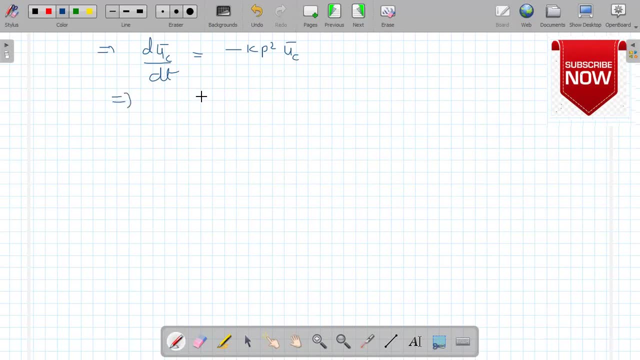 So we do the variable separation and then integration so that we have: the value of uc bar is equal to c raised to the power minus kp square t, Putting t is equal to 0. we have uc 0 comma t. sorry, p comma 0 is equal to c. So we need this value. We use the, we take 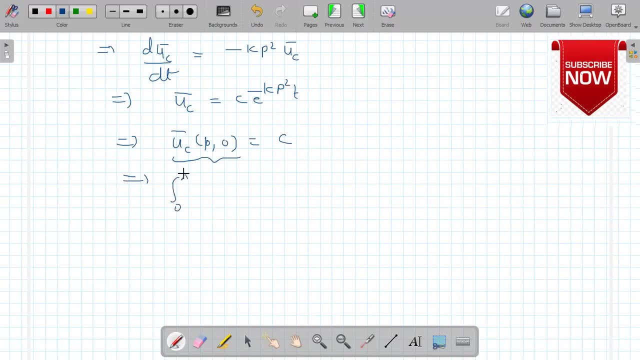 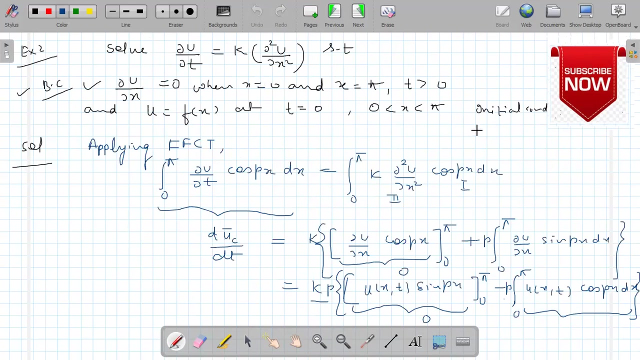 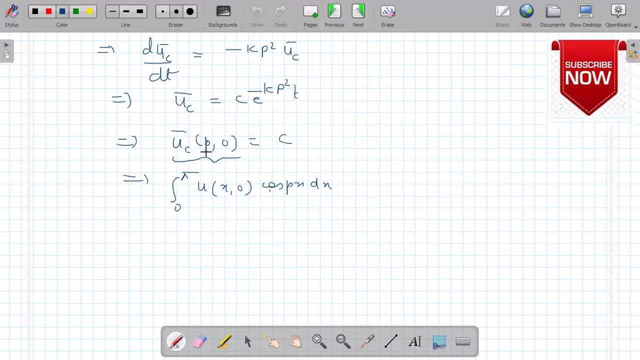 this. we write this as an usual form, which is 0 to pi. u, x, comma, 0, dx, cos, px. either you can take this condition of finite Fourier cosine transform or you can convert this condition into its definition, because this is a finite Fourier cosine transform. This is a normally accepted definition of the linearięc, Because this is a finite Fourier cosine transform. we will also take this as the final solution, because if you want to convert this to the linearięc, then you need to take this as the final solution. and let us report the previous. 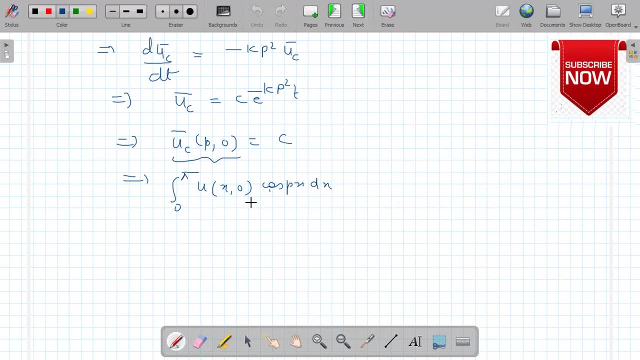 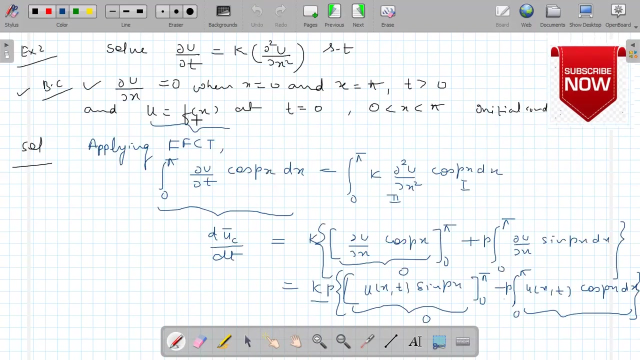 Fourier cosine transform of the function ux comma 0, whose notation is this. So we are writing this in its original form And ux comma 0 is given in the question. ux comma 0 at t is equal to 0, means ux comma 0's value is fx. 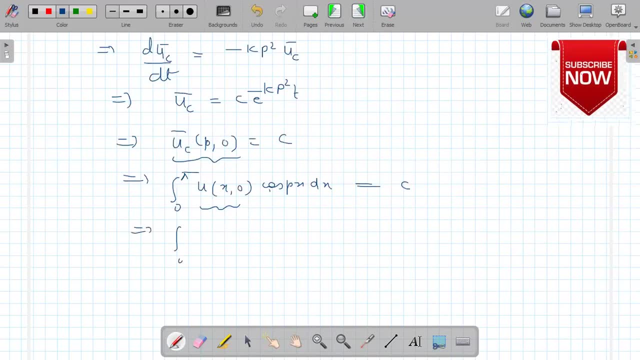 So here we can write fx. So this is the value of c. So this value is the equation number of c. Here we call it 2.. Let's call it 2.. In equation number 2, the value is c. 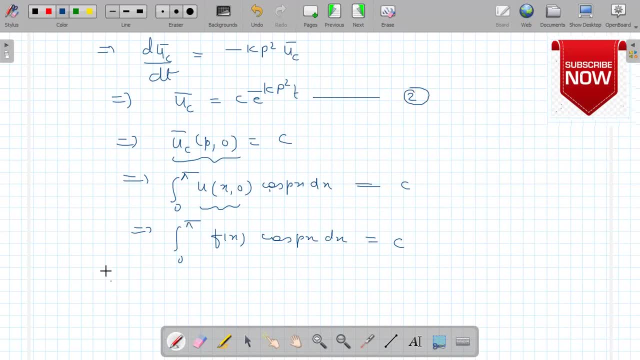 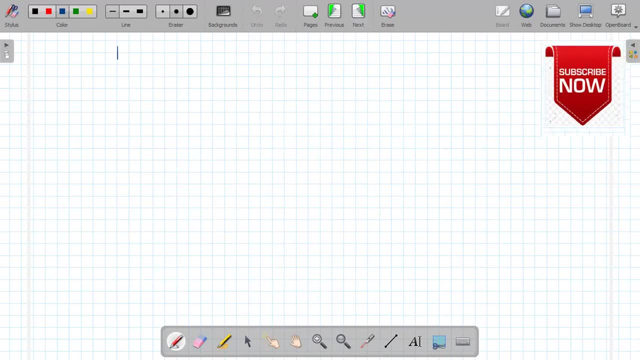 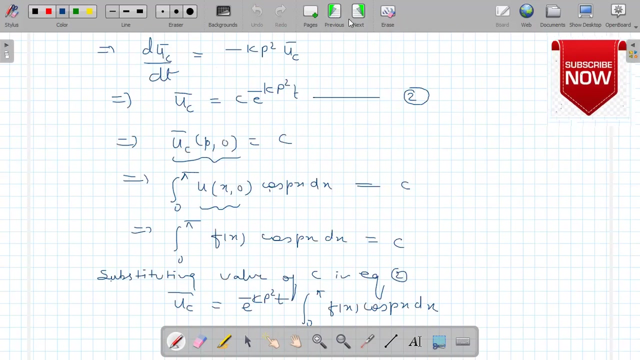 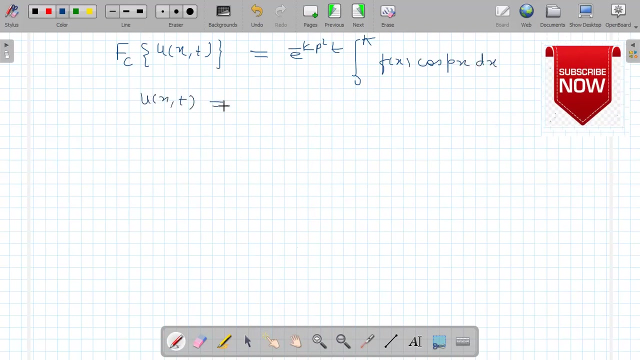 Now the next step is because uc bar is nothing but Fourier cosine transform of ux comma t. Okay, Let me write the whole expression: fx, cos, px, tx. So ux comma t is Fourier cosine inverse of this expression, Which is equal to. 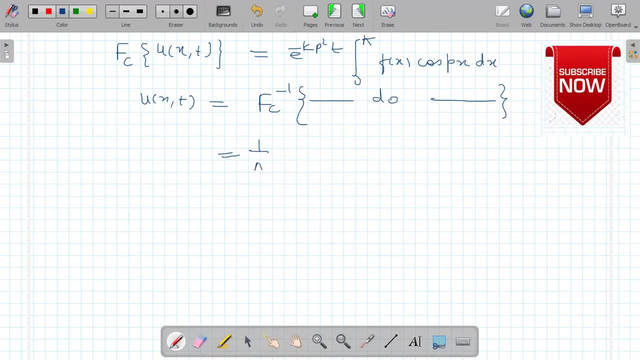 1 upon pi. uc bar at 0 comma t, uc bar at 0 comma t plus 2 upon pi. This is by definition. I am writing. You should look at the definition again If you don't remember the formula: uc p, comma t. 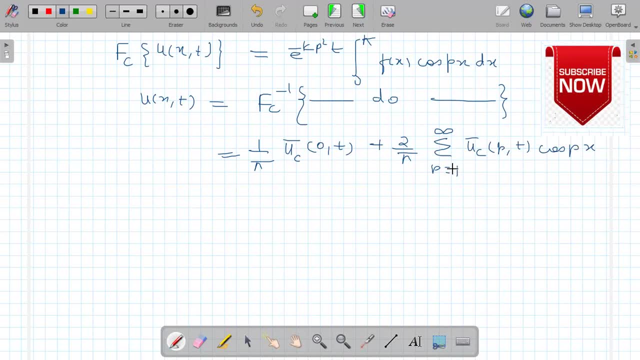 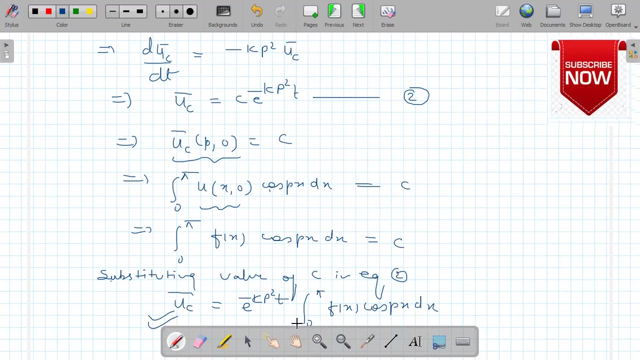 cos px, where uc at 0 comma, t is 0 to pi us comma by definition. you, you, so this is given to you as FX DX, so you can replace this in this expression by this expression, and this UCP for Marty is replaced by this expression. okay, so?